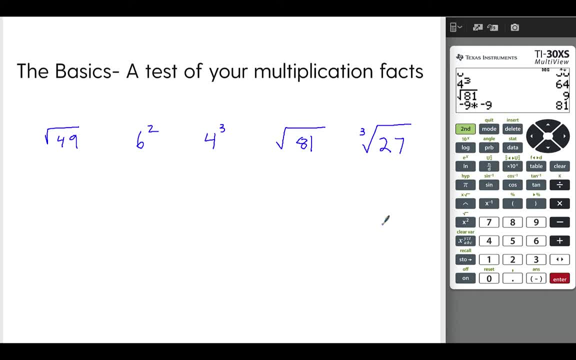 before you spend time trying to memorize your multiplication facts if you still don't know them. The first six questions you can't use a calculator, so you will need to know your multiplication facts, but the remaining 40 you can use a calculator. And so for that reason, if our goal is to just pass the GED, knowing the 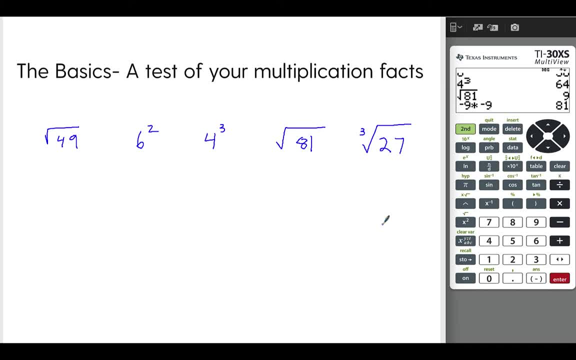 calculator, I think, is more important, So I always encourage students to use it. If you want to focus on your multiplication facts, that's a very worthwhile will help you a lot in life. That's not what this video is about, though, so I'm gonna kind. 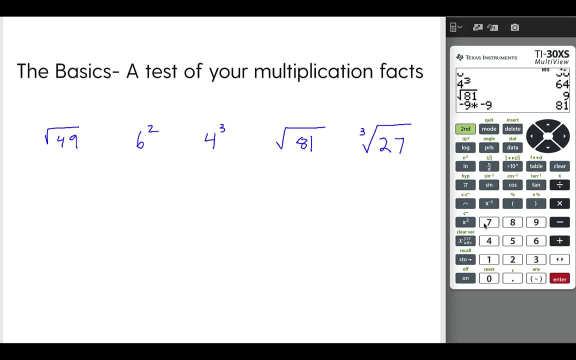 of just go over those. You can also show you on the calculator. So this is a question to you: What number times itself is 49?? What number times itself is 49?? And I'll tell you: the answer is 7, because 7 times 7 equals 49.. Keep in mind, though, so does negative 7. 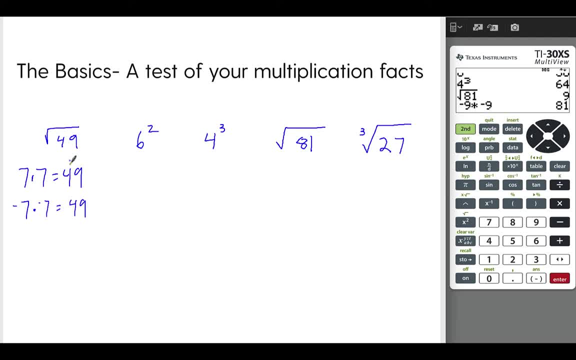 times negative 7.. So there's actually two answers here. It could be 7 or negative 7.. So let me go ahead and show you how to how to enter this in on the calculator. So you've got second here to get this green radical sign. So notice I. 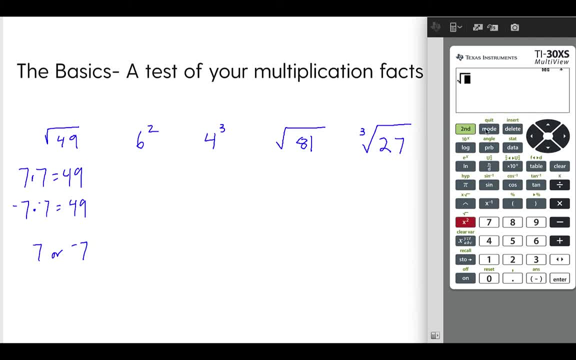 hit the second button, it's red. and now I've got that And we can put 49 in here. The calculator is only going to give you one answer, but if you do negative 7 times negative 7, you will get 49.. Okay, this is 6 squared. So what this is is 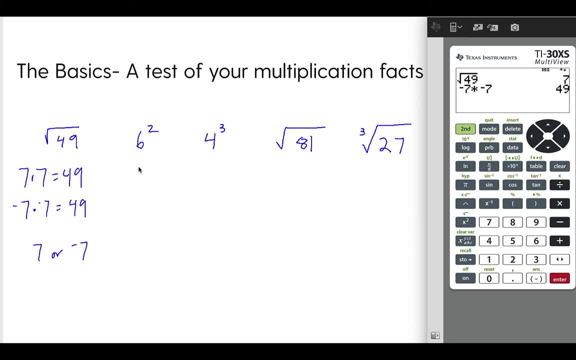 what number? what is the answer? if you take 6 times 6, or six times itself, So 6 times 6 is 36.. Okay, keep in mind here. What if? what if we had negative 6 squared? And we actually mean by negative 6 we mean the whole negative 6, like this: 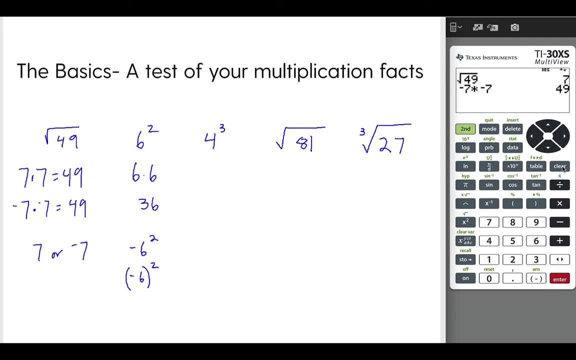 So if you just do, look what happens over here on the calculator- If you put in negative 6 and then you square it, hit enter, you're gonna get a negative number and that's probably not the answer you want, because really what you want this: 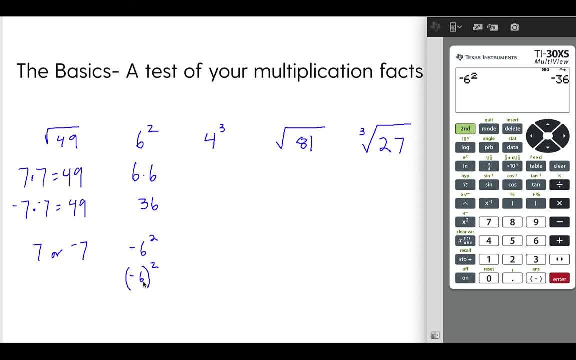 often comes up in, like the quadratic formula, for example. what you want is you want to square negative 6, so you have to use the parentheses- negative 6 parentheses- and then square that. then you get the right answer. because this first one- we have negative 6 squared with no parentheses. I'm here in the 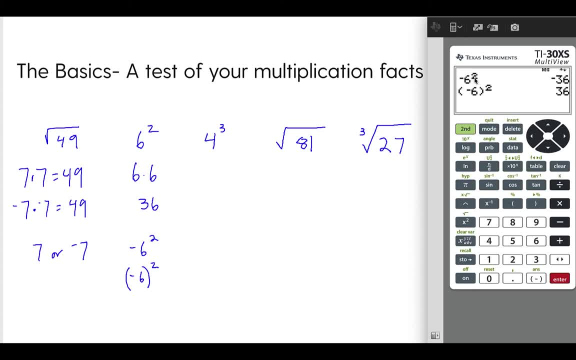 calculator. this is following PEMDAS. it's squaring, so it's getting 36 and then it's multiplying it by a negative to get negative 36. so you have to put the parentheses in to kind of tell the calculator. here's the order by which you. 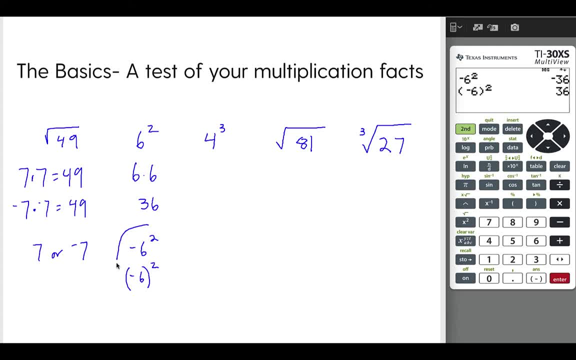 should do things, so keep that in mind. I have seen this, this type of thing, come up on the GED. so 4 to the third. this is a question to you: what? what is the answer if you take 4 times 4 times 4? so let's do the calculator first. this time you can do 4 here. this. 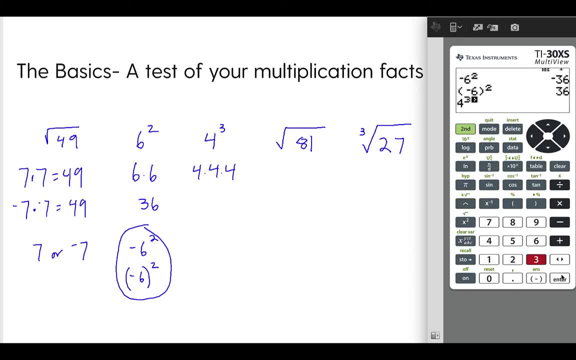 little upside down V. that's the exponent sign, so you could put a 3 in here and the answer is 64. square root of 81 is similar to this one. it's going to be 9 or negative 9. so again, if you take negative 9 times a negative 9, you're. 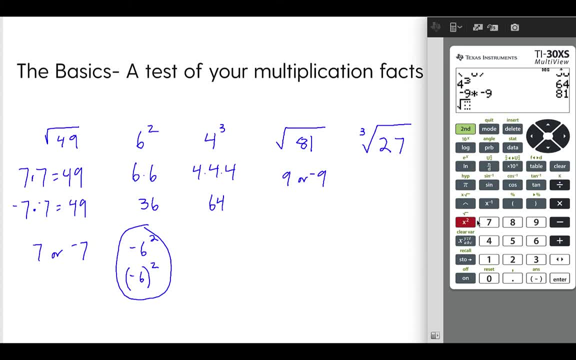 going to get 81, but if you just do the square root of 81, you only get one answer. but negative 9 also works, and so for this reason, testmakers like to formulate questions where they want to make sure you know the negative is also a potential answer. so keep that in mind. 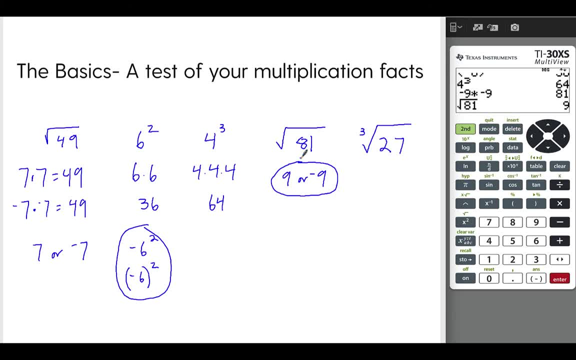 let's do 3, sorry, the cube root of 27, that's how you would say this one. 3, the cube root cube, is denoted here by the 3 and then the root is the: here's your root sign. so this one is a little tricky. so oftentimes 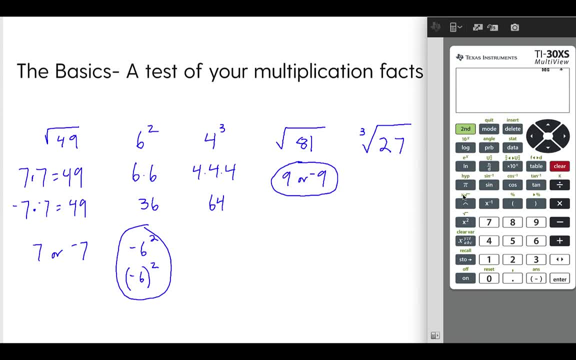 if I get students to want to do so, here it is. it's the X. they want to hit this first and notice it gives you an a and s that stands for your previous answer, and that's not what you want. so what you have to do is enter in the three: first and then second and then. 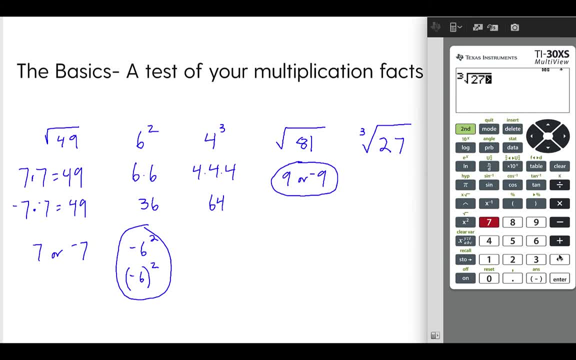 this button, then you put in 27. so this is what number times itself. three times is 27 and the answer is three: 3 x 3 x 2: 3 is 27.. So the answer is 3.. Okay, so here's all the answers. Let's go ahead and back and circle. 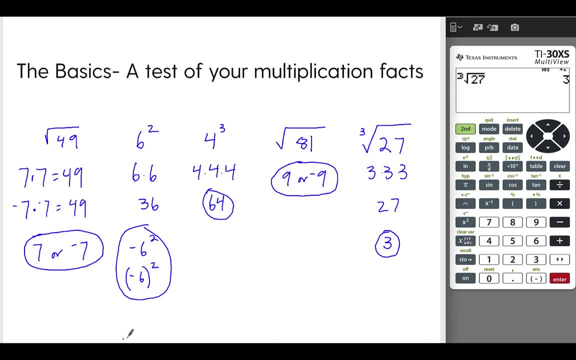 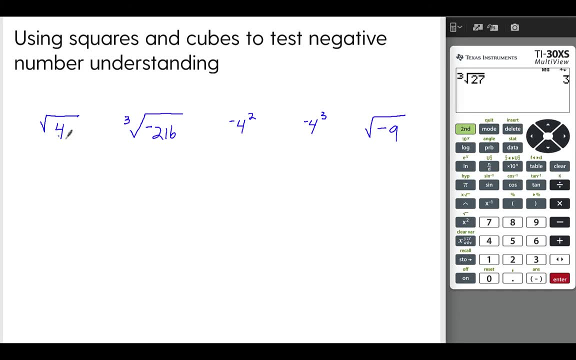 them All right. So using squares and cubes to test negative number understanding. So again you have the square root of 4.. This could be- oh, not that square root. The answer could be 2.. 2 times 2 is 4, but so is negative 2.. What is the cube root of negative 216?? So what number times? 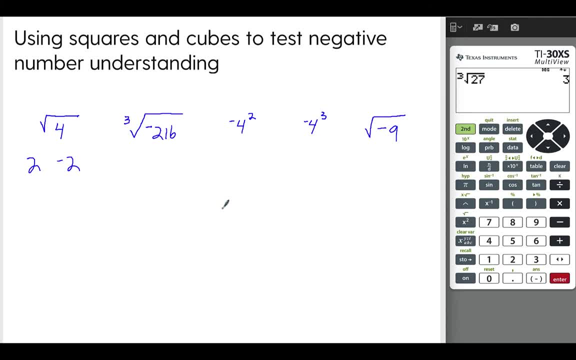 itself 3 times is negative 216.. You could put this in a calculator. If you want to do the 3 first, you need to do the 3 first. Then you could put in a negative 216. And you'll see the answer. 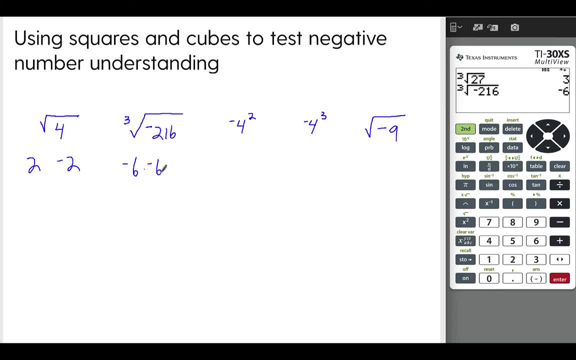 is negative 6.. Negative 6 times negative, 6 times negative 6.. So when you take negative 6 times negative 6, you're going to get positive 36.. Drop down this other negative 6, and that's what makes it back to being a negative, And so your answer is negative. 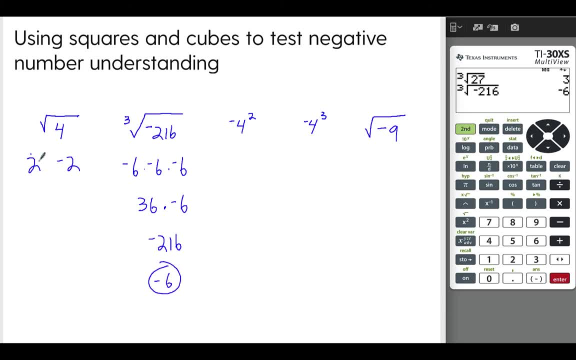 6. Okay, All right. So a negative 4 squared- remember- 4 times 4 is 16, and negative 4 times negative 4 is also 16.. All right, So if you take negative 4 to the third again, this is the same as taking negative 4 times. 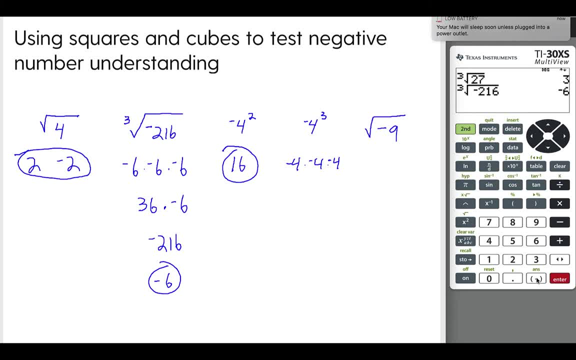 negative 4 times negative 4.. You could put it in the calculator Again. I would put it in parentheses: Negative 4, and then exponent 3, and you'll get the answer is negative 64, which is correct. Now, this is a precarious one. What is the square root of negative 4?? 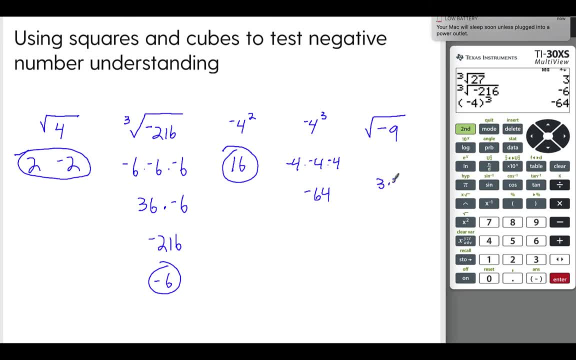 Negative 9.. So, if you remember, 3 times 3 is positive 9.. That doesn't work. Well, what about negative 3? then Negative 3 times negative 3 is also positive 9.. Hmm, What if we take negative 3? 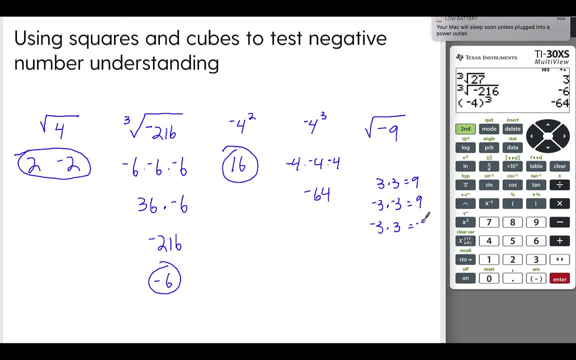 times positive 3?? Sure enough, that will get you negative 9.. But guess what? Negative 3 and 3 are not the same numbers. You can't do this. This is not what this is asking. This is asking what number. 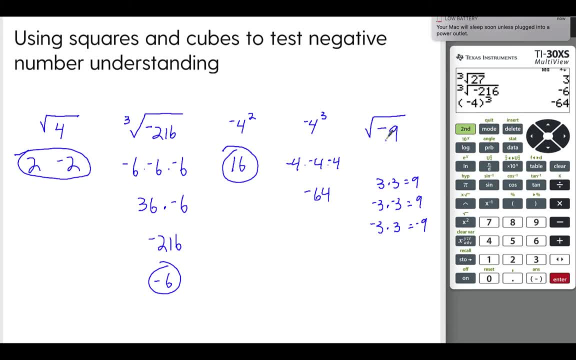 times itself is negative 9.. And the answer is there is no solution or it's undefined, And test makers like this, They like this a lot, And so you want to be aware of this and be on the lookout for it and don't get tricked by it, And also know what this undefined is. I always tell. 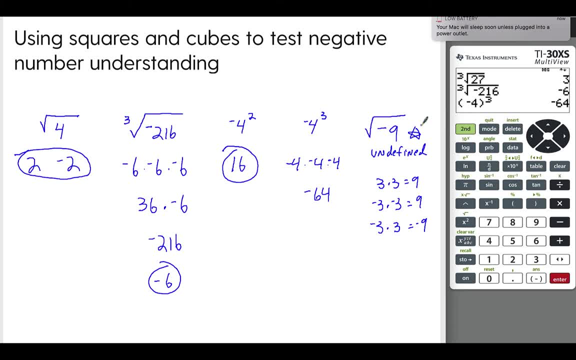 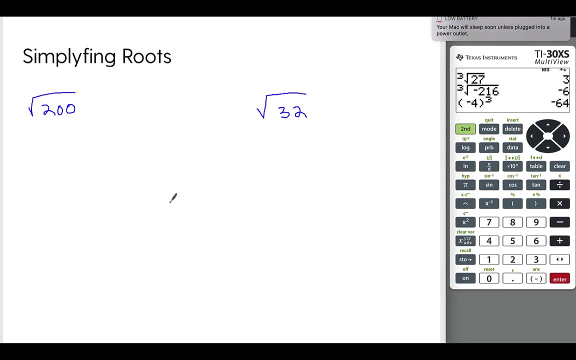 my students. undefined is just a mathematical term for weird Like it's possible, like in math, we can write it, but there's no solution to it. Doesn't really make sense. So that's sort of what undefined means. All right, And so every now and 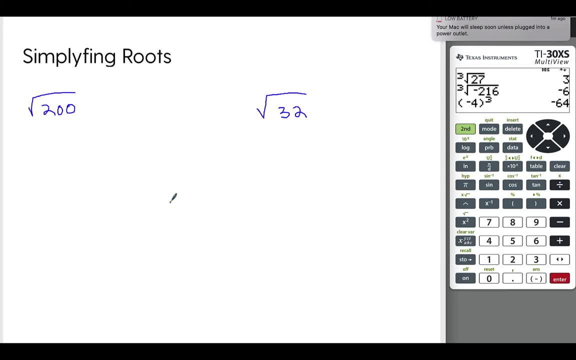 then I see, especially in GED books, simplifying roots And the square root of 200.. Well, if you put, if you have a calculator and you put the square root of 200 in the calculator, you're going to get- well, they actually do it for you- 2 to the square root of 10.. And so how do they get? 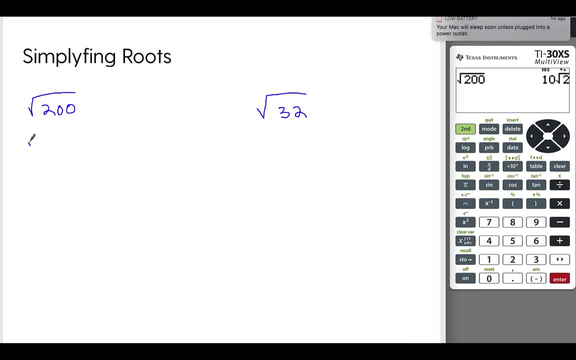 that What we're doing is is you can actually break these apart. We know how many ways can we make 200, right, We could do 100 times two. we could do 25 times eight. So if you do 100 times two, that's the. 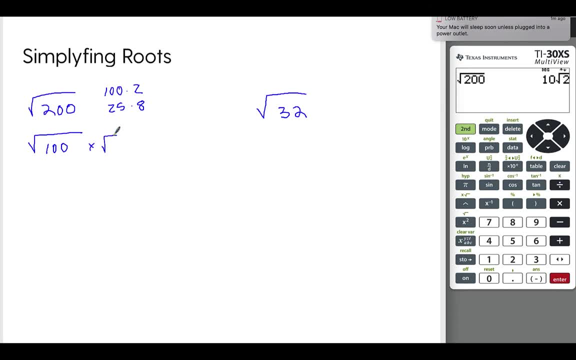 same as taking the square root of 100 times the square root of two, And if you take the square root of 100, that is 10.. And then we have this 10 square root of two. If you were to take the square root of 25 and eight. 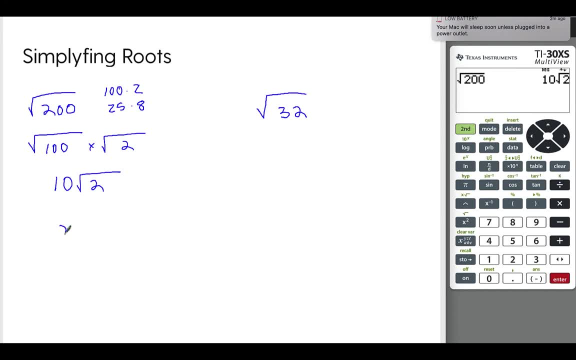 Okay, so if we do 20.. Square root of 25, times the square root of eight? Well, the first thing is that there's a square root of eight embedded in here. We could do the square root of 25, and then we can break the square root of. 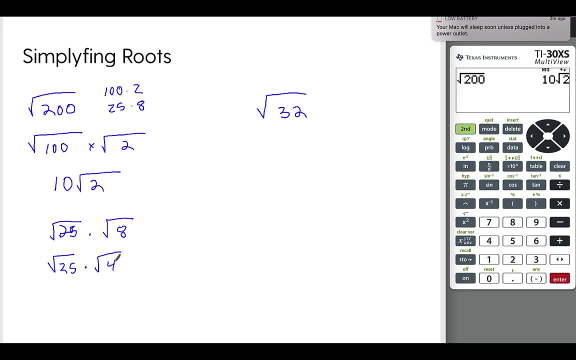 8 up into the square root of 10.. root of 4 times the square root of 2, and these happen to be perfect squares- 25 and 4, so the square root of 25 is 5 times the square root of 4, which is 2. 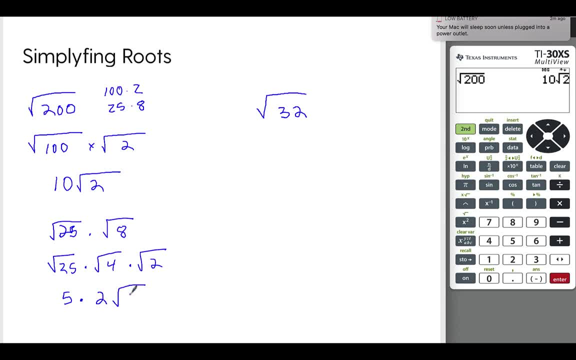 and then this is as far as we can go here. so what's 5 times 2? it's 10, 10 times the square root of 2, so two different ways of getting the same answer. so this, to me, and for most of the students that I work with, this is a. 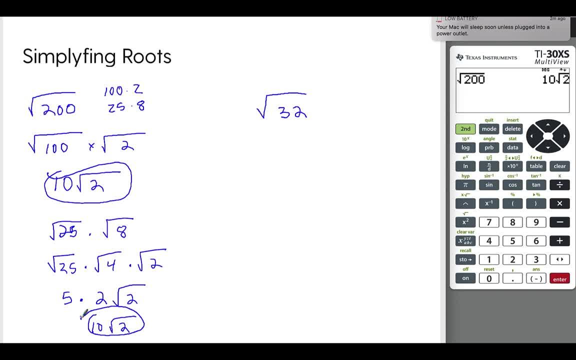 fairly advanced situation advanced topic. I really encourage students to understand the calculator and I really encourage students to know the basics of cubing and squaring and exponents and things like that. this, I would say, is a little bit more of an advanced topic if you're, if you know, you've been fighting. 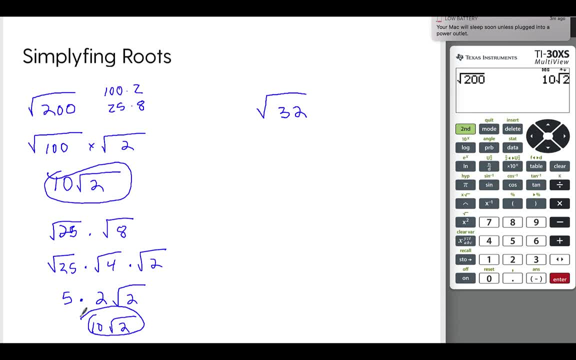 to get that 145. this can push you over if you're in the 130s or low 140s. I think there's easier stuff for you to learn. that being said, let's continue. here we have the square root of 32, which, if we think, how many ways can we get 32? well, you could do 16. 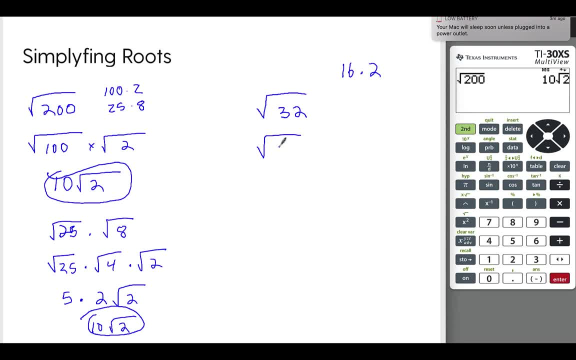 times 2 and 16, square root of 16 happens to be a perfect square, because what number times itself is 16. it's 4: 2 times 16 is 4: 2. we can't go any further, and so there's your answer. 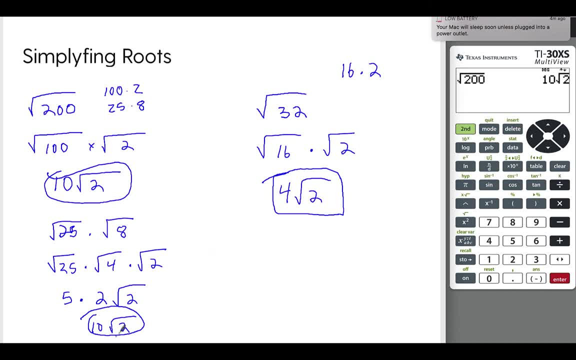 ok, let's do one more. all right. so this one is set up as a fraction: the square root of 32 over the square root of 2, so keep that in mind. you could also think of it like this: the square root of 32 over 2.. 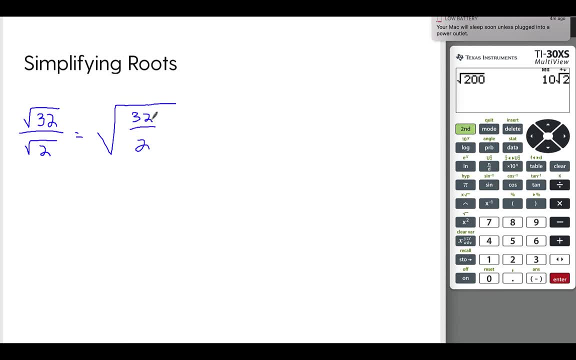 over 2.. How many times is 2 going to 32?? Well, if you've got to use a calculator, go ahead, No problem. 32 divided by 2 is 16.. So now you have the square root of 16, which we just